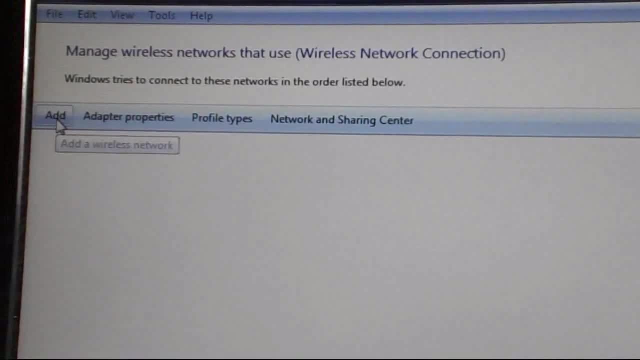 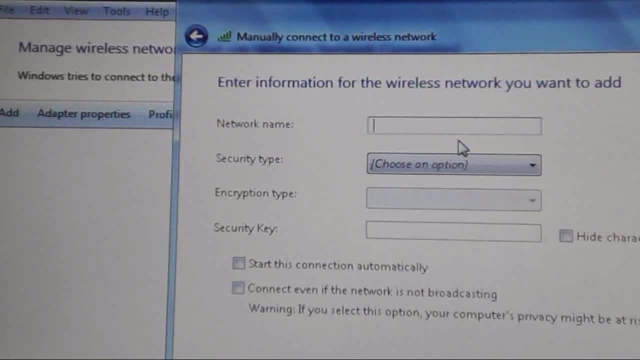 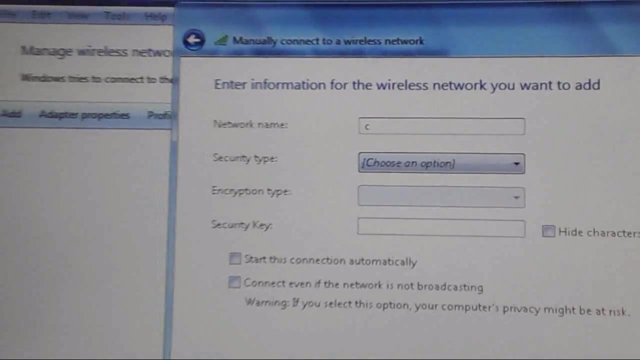 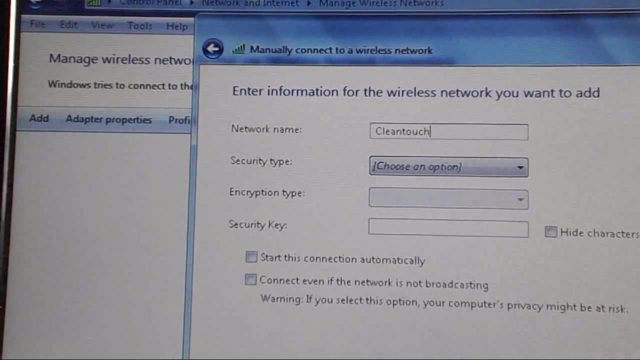 to add the new network Wi-Fi network to your laptop or desktop. Just click on add and check down manually. create a network profile- this first one, okay- and you have to type your network address correctly. For example, I have here, like clean touch, Don't be miss-spling here and miss-tap that spilling, just tap the correct. 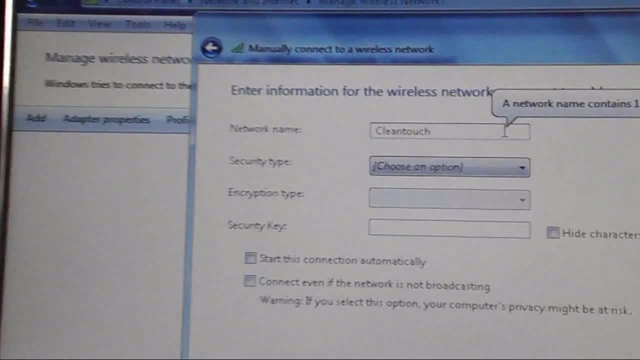 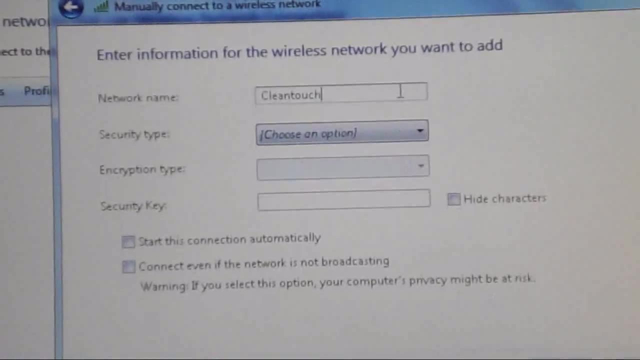 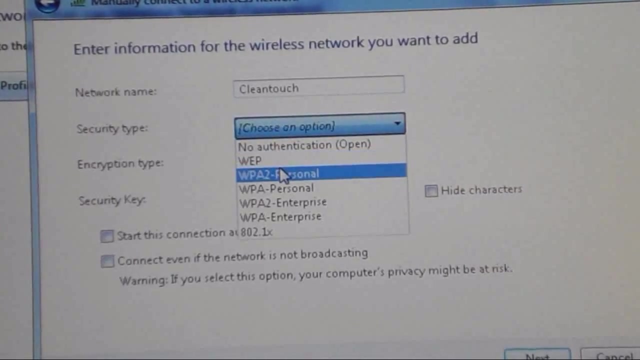 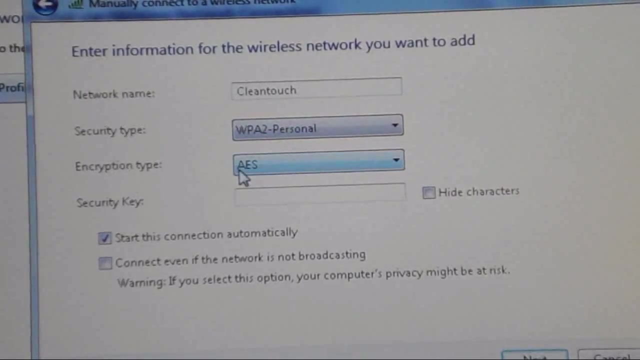 network address. here, For example, I have that clean touch here and later. and in the next box, here, the security tab, you have to choose the WPA2-personal, this one, and this will let me cover in different type AES, and here you have to tap the password of Wi-Fi. 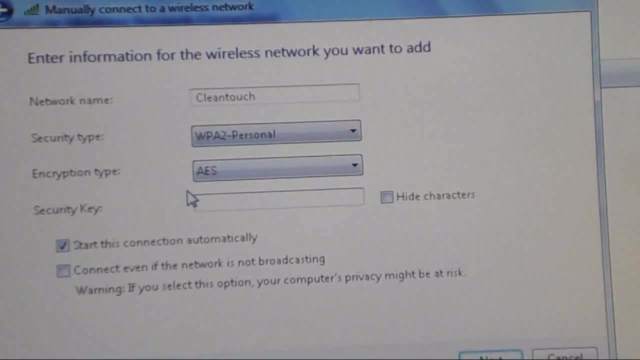 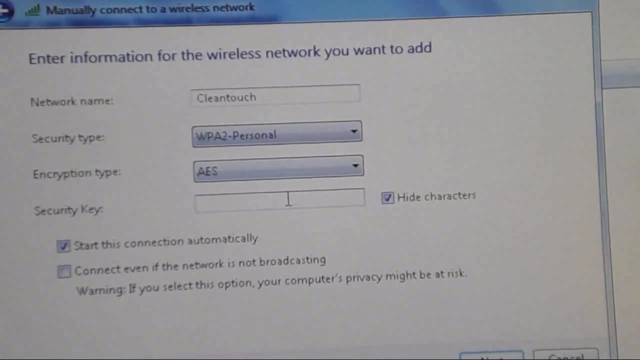 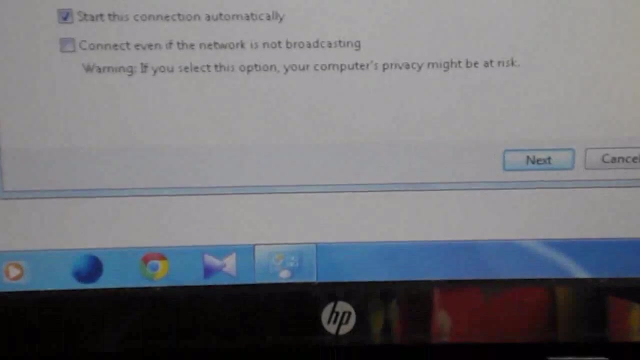 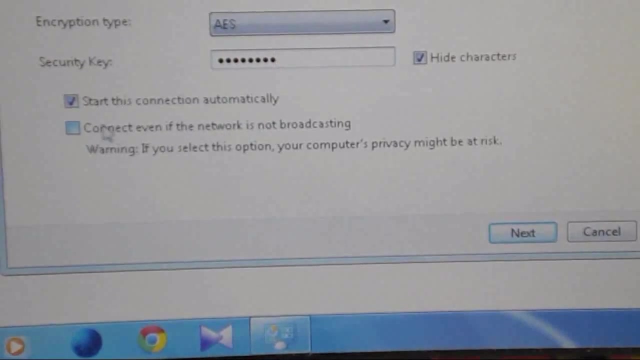 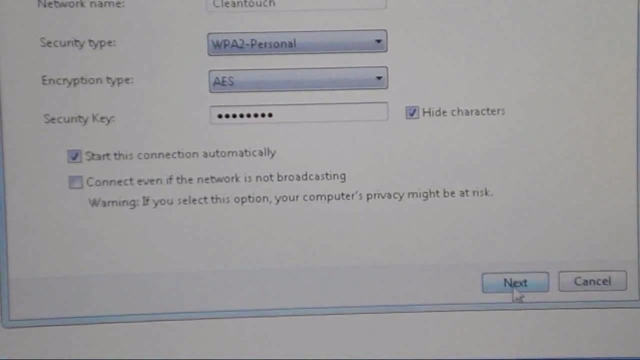 So I'm going to tap the password. Okay, so done. Here you can see two more option here. You can start with this network connection automatically or connect you on. if the network is not broadcasting, you have to start this connection automatically and just click on and click on next. 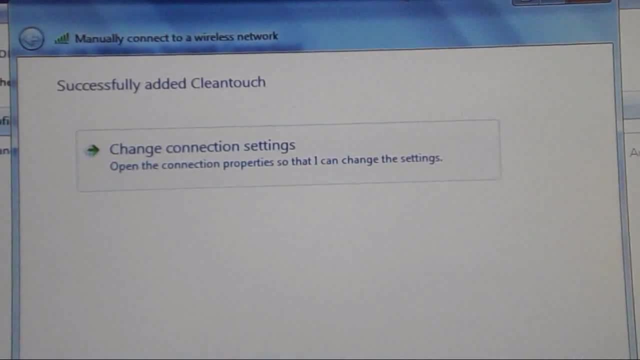 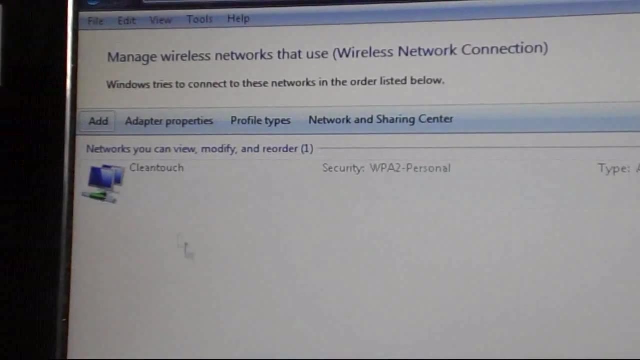 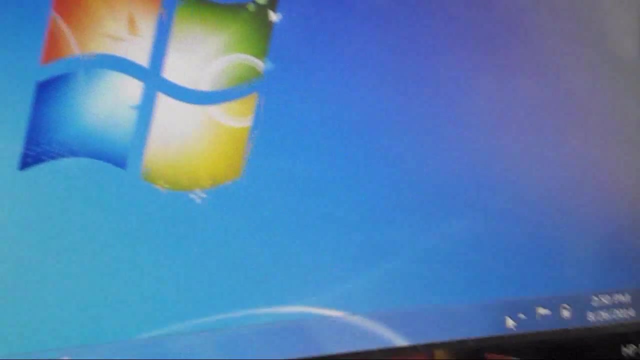 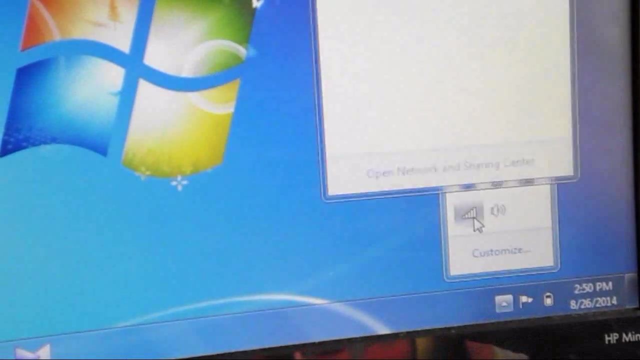 okay, done. it has successfully added to your my laptop. let's close it. and now you can see here: now network icon, click touch and now it's connected. let's see here, in the tab where you can see there the network option here, just click on, double click on that, just click on it. 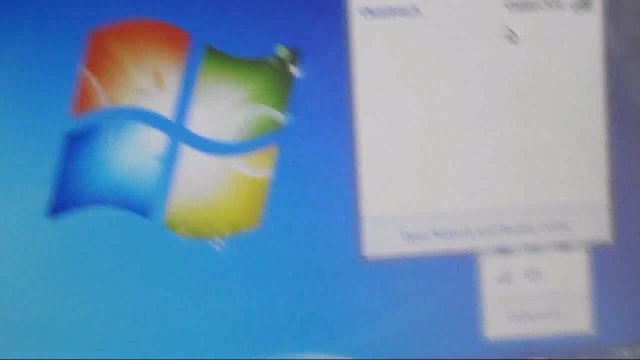 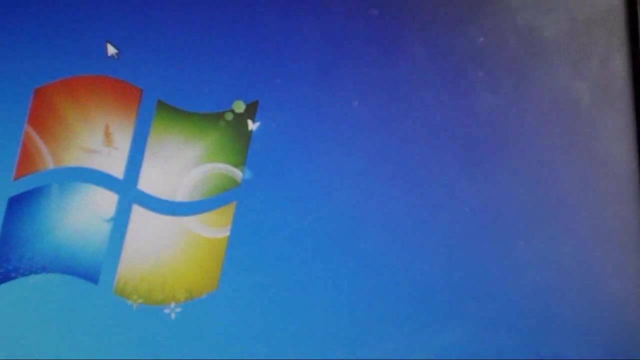 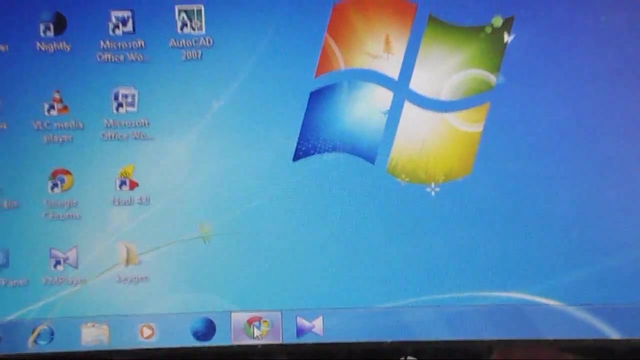 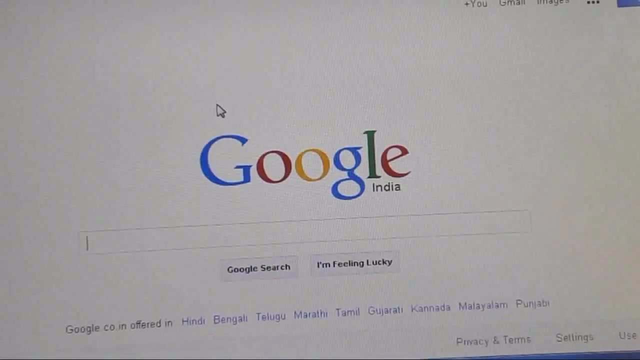 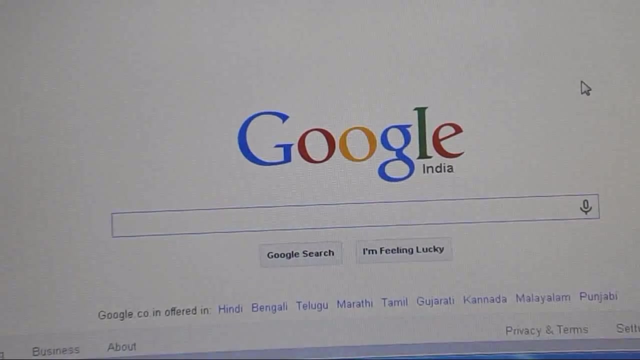 look at that. here is showing that connected. you can see here the network connection is showing that showing the connected. now let's check the internet. look at that. the internet is on now and the Wi-Fi working. fine, it is not right now, so like that you can connect your laptop or a network easily to Wi-Fi. use the.